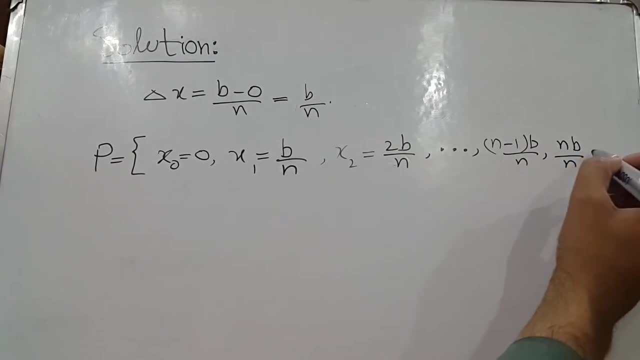 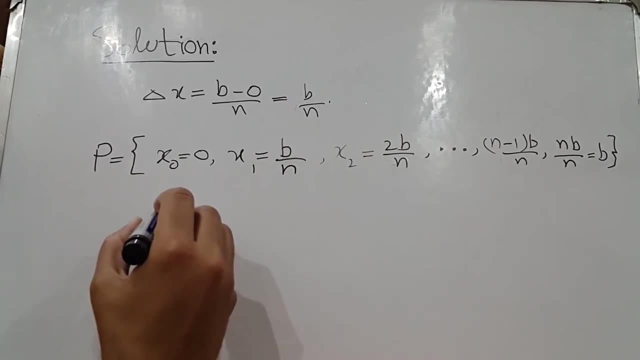 And the last point is n by n, which is equal to b, Ik is equal to kth interval k minus 1 by up to. Thus mk is greater than or equal to n sine of f in the value of xp. Hence a particle is equal to celestial and the integral of xp into an Xpам. the equation: 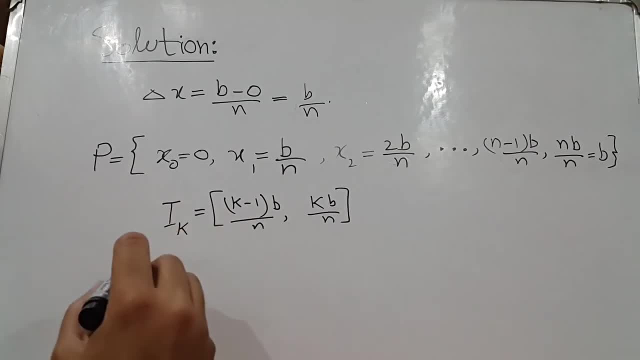 will have advantageous relations, And we will. about this answer in next class With respect to function of mk. here we have have the objective expression of respect to volume s around xprier. You can see that, firstly, God 26 walk down to here and Zumtow bounce out of this function. 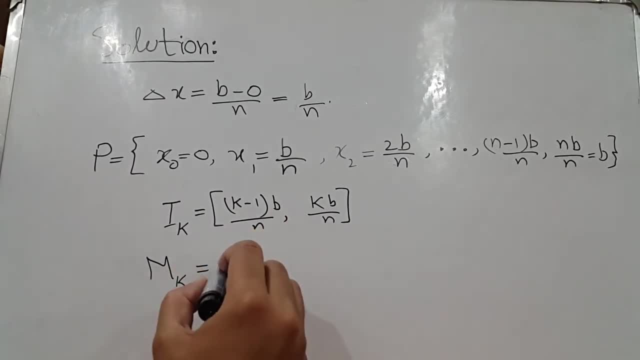 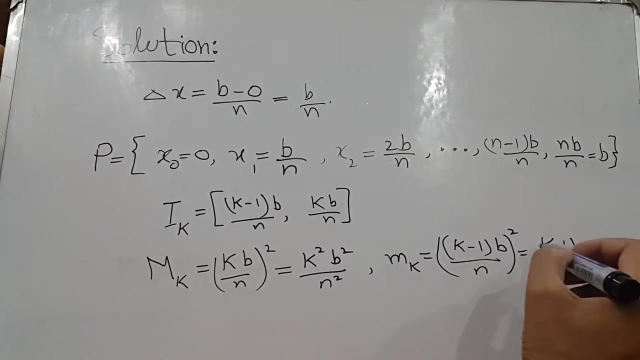 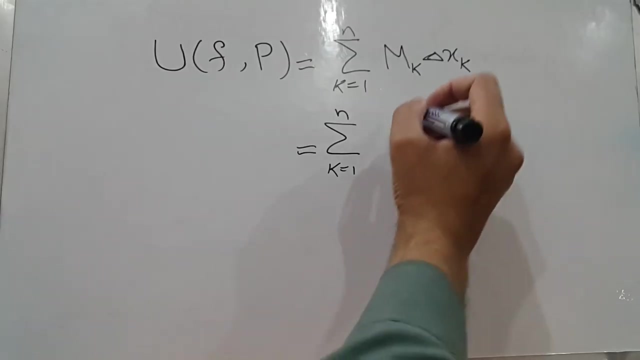 mk is equal to kb by n whole square, which is equal to k square. b square. divided by n square mk is equal to k minus 1 b by n whole square. this is equal to k minus 1 whole square. b square by n square. the value of upper sum is putting of the value of mk. 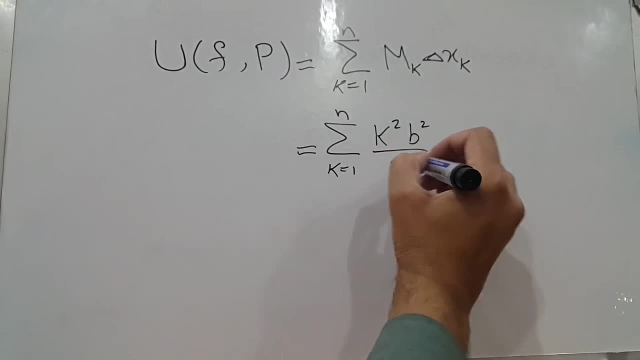 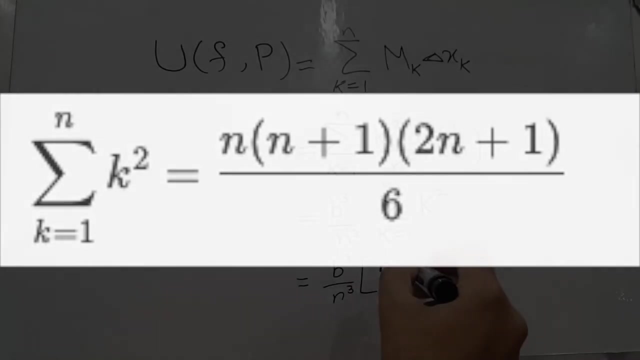 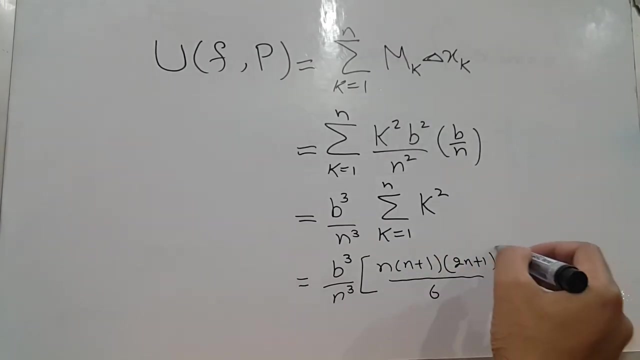 k square. b square over n square into the value of delta xk is b by n. this is equal to b cube by n cube. summation k varies from 1 to n k square. this is equal to b cube by n cube into n plus 1, into 2, n plus 1 by 6, you get n plus 1, 2, n plus 1, 6 n square b cube. the value of 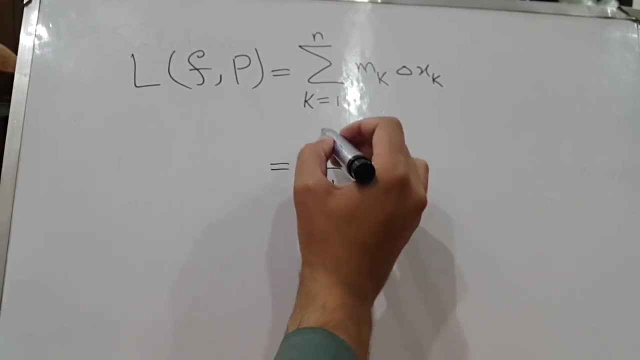 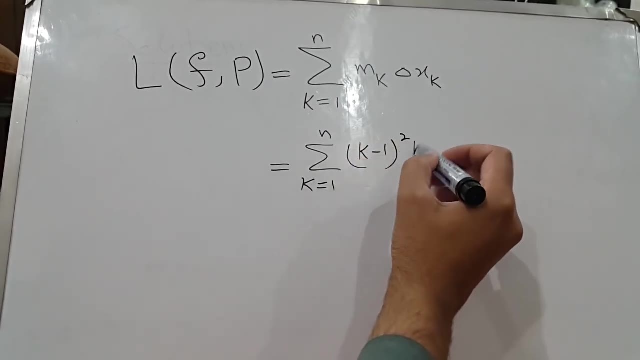 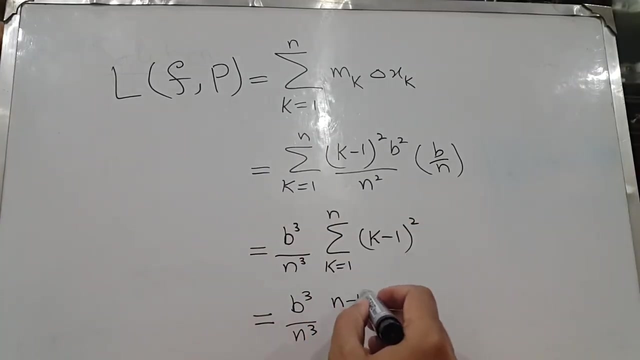 lower sum is: summation k varies from 1 to n. k-1. whole square. b square over n square into b by n. this is equal to b cube, n cube. summation k varies from 1 to n. k-1 whole square. b cube over n cube n-1. 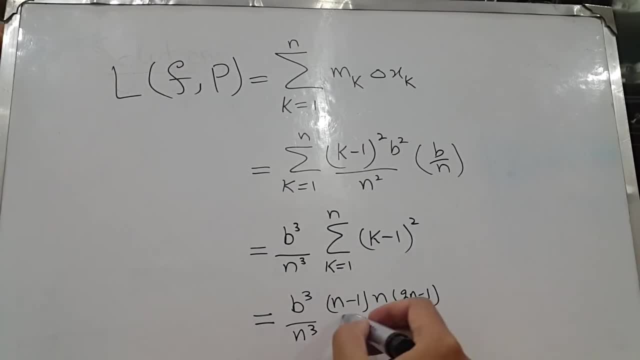 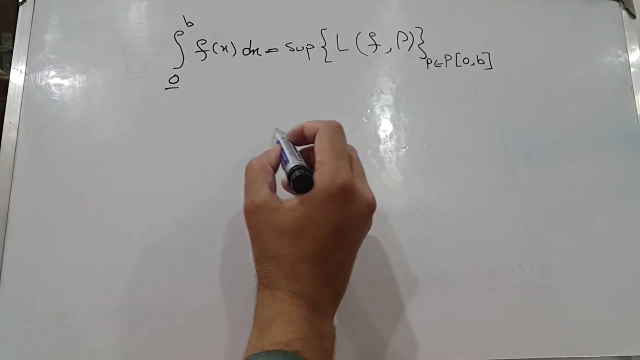 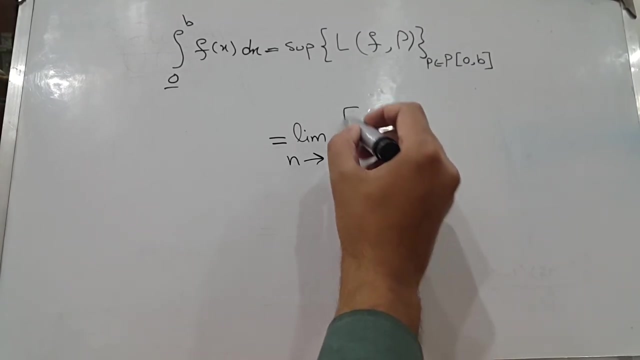 into n- 2n-1 divided by 6- 2n-1, 2n-1 divided by 6n. square b cube, the value of lower is equal to integral, is equal to limit. n approaches to infinity: n-1, 2n-1. 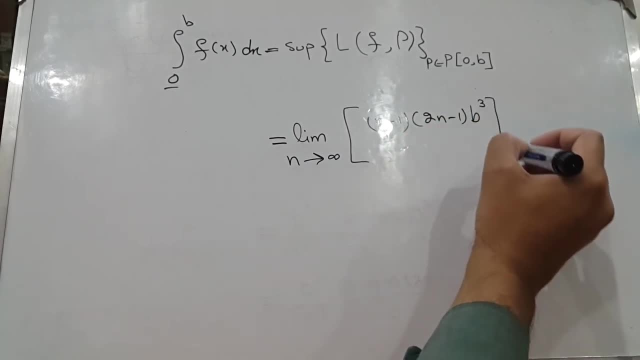 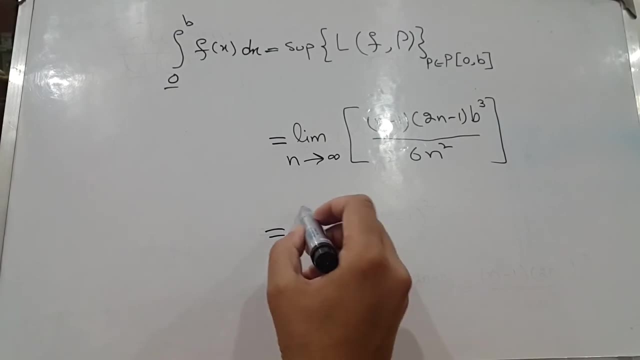 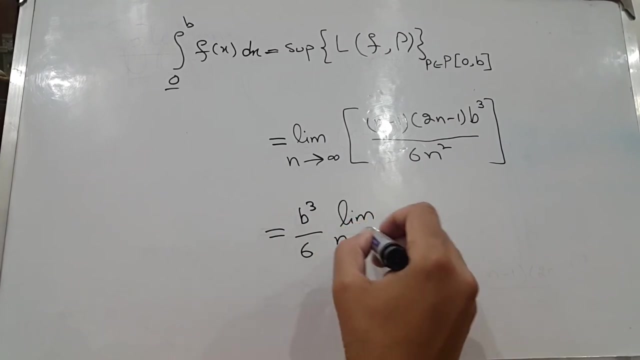 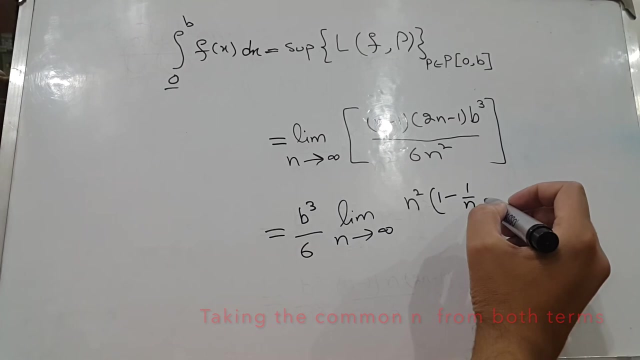 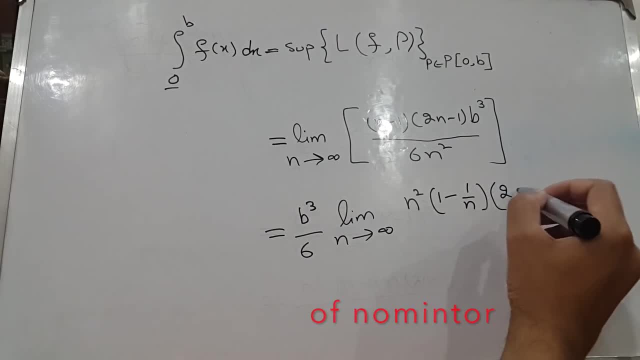 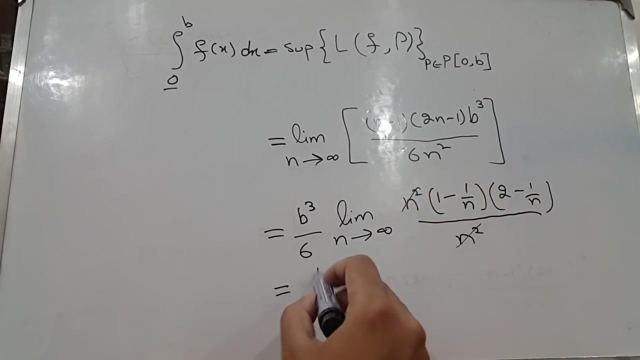 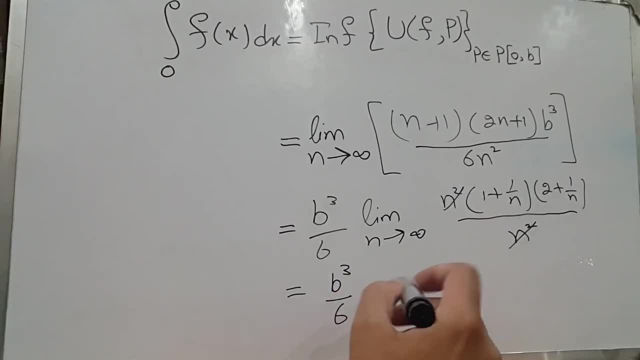 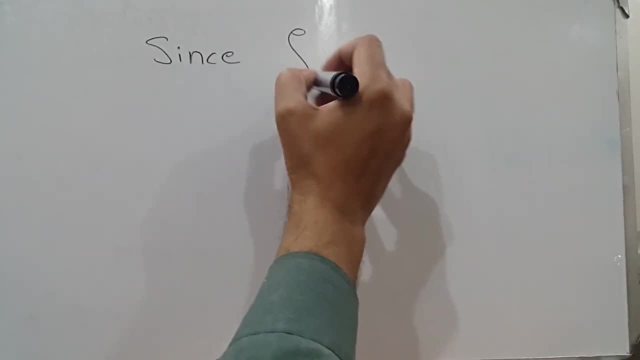 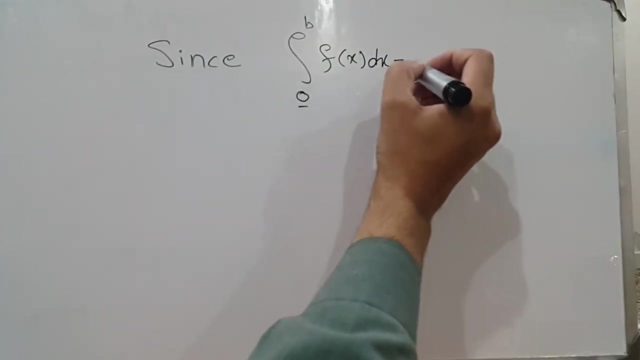 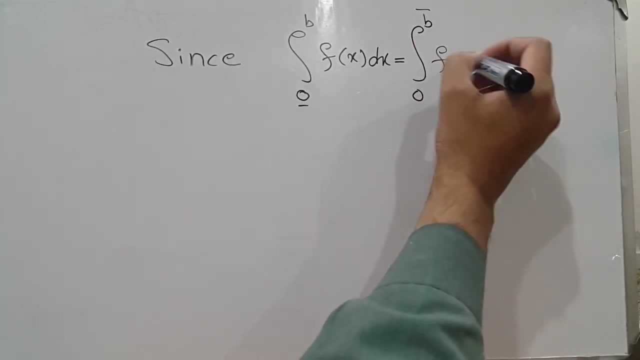